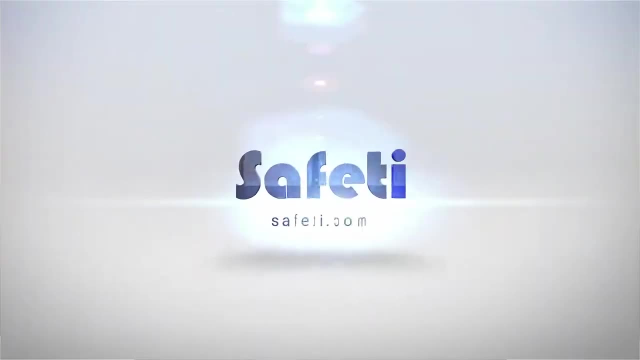 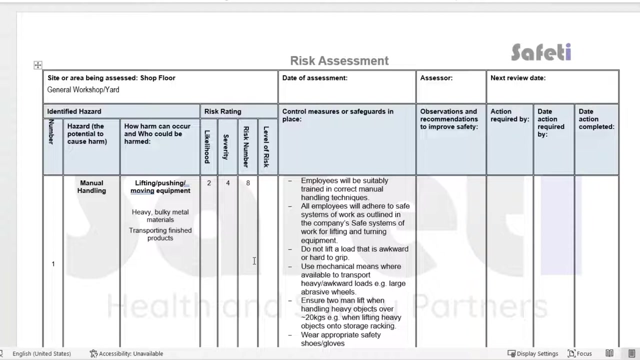 Hey there, and you're very welcome to our shop here at safetycom. I wanted to give you a quick run through as to what's included in the workshop risk assessment pack. So we've really piled in the value here, or at least attempted to, and so I want to just describe to you exactly what's. 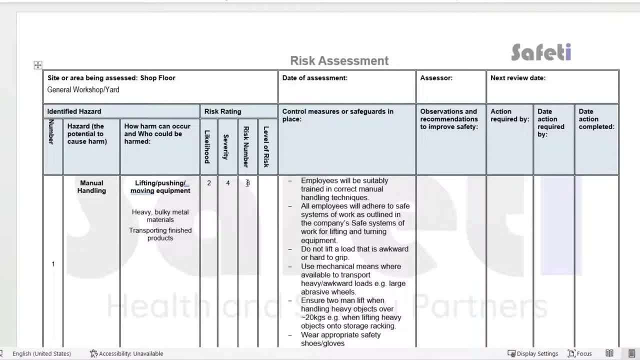 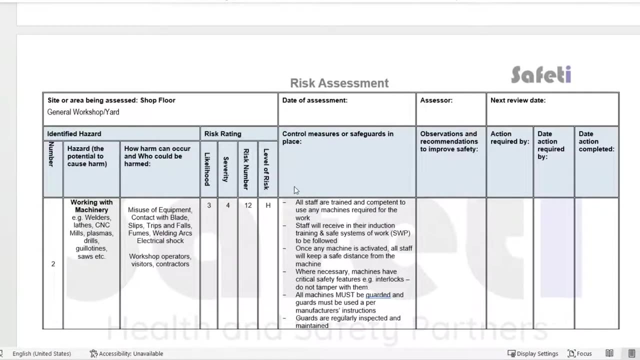 included in this product at this present moment in time. So, first of all, you have one of the most detailed risk assessment examples we have, which is the workshop risk assessment. As you can see here, it's detailed. it's using another one of our templates, which 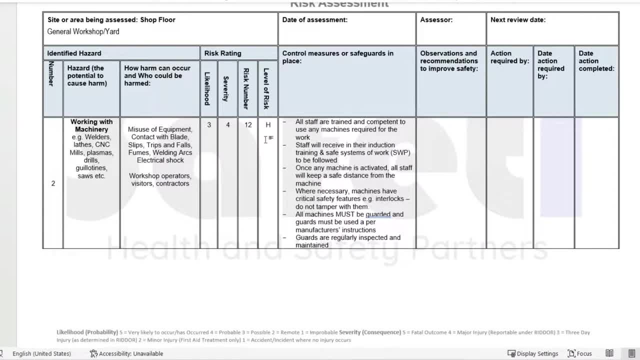 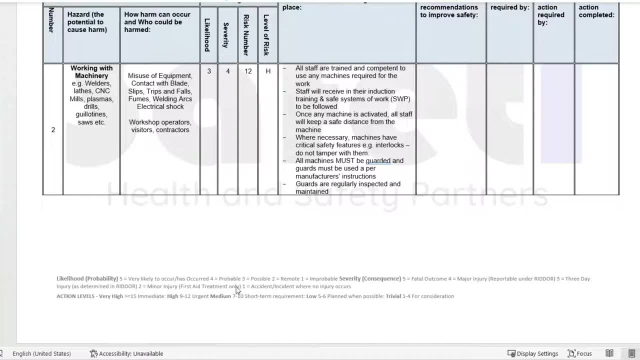 we feel is quite user-friendly and gives you lots of opportunity to put in your control measures. There is some guidance around how to judge the risk level there and, as I said before, if you haven't taken our risk assessment training course, which is completely free, 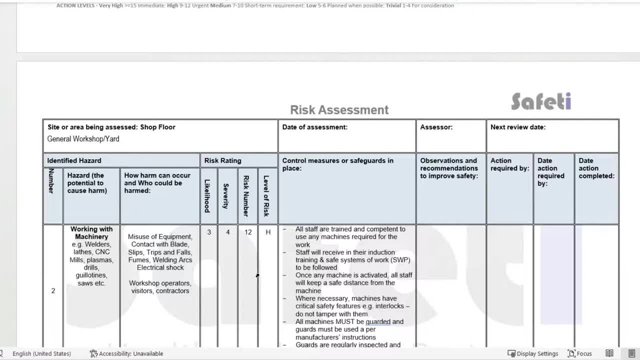 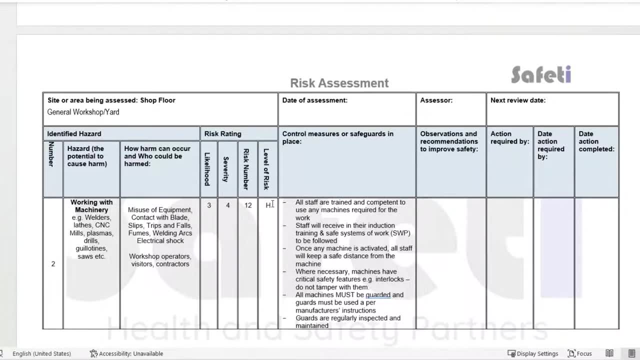 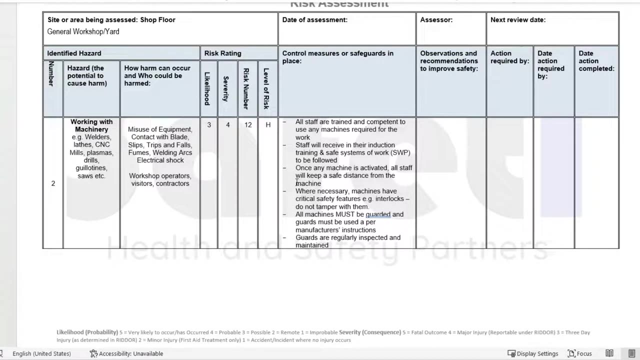 and you want a bit of help with that, then please do so and please go ahead and send that over to those in your organization who might find it useful. So, as I say, as you can see lots of detail here around workshop typical risks. This is a general risk assessment that would feed into 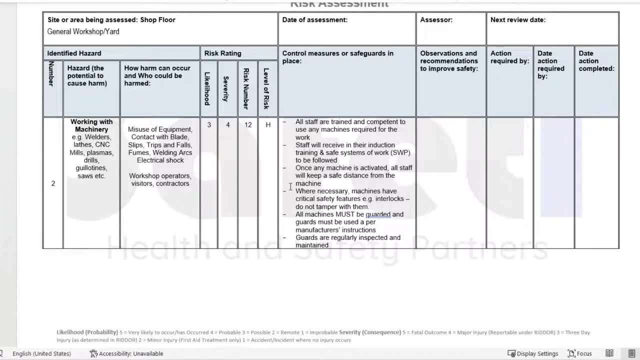 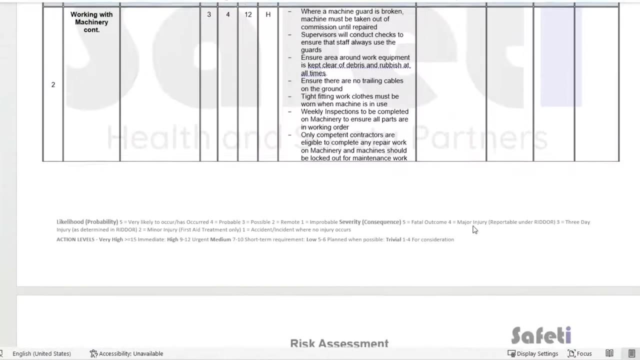 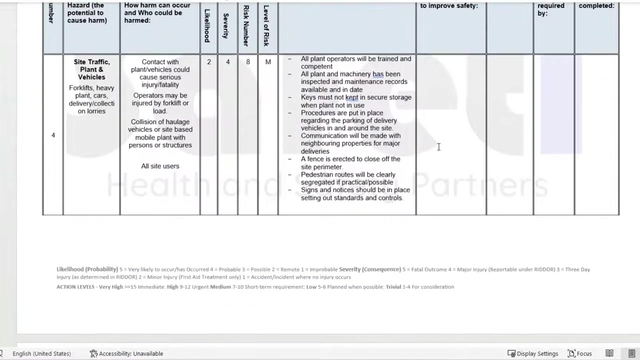 more specific stuff like safe work procedures and specific equipment. risk assessments were necessary, which we'll touch on shortly. As you can see here workshop machinery and it is outlined and there's a couple of pages of actual control measures there that are relevant across the board. We have a section on cost or control of hazardous substances site traffic. 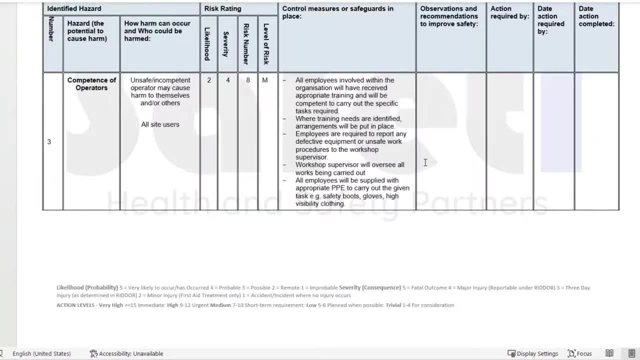 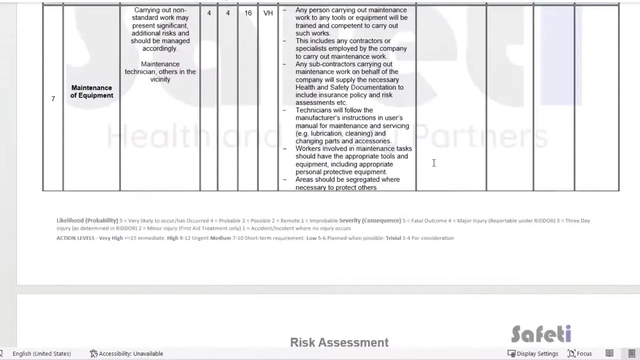 plant and vehicles for the movement of plant and so forth. Competence of operators, which is always a big thing, an important aspect, making sure you have the right people doing the work, and everything that goes along with that. Okay, so it goes on and on. and maintenance as well, covered there as well, and welfare and waste. 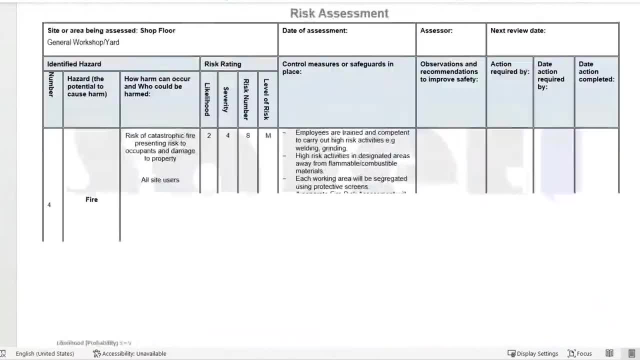 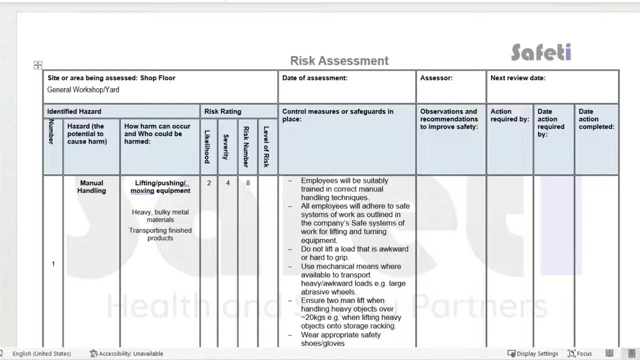 management and so on. So we've got 11 pages in that example. As I said previously, you know we're not trying to necessarily cover everything with these examples, but it should give you a very good start to making a site-specific risk assessment, which is, of course, the end goal here. We've also 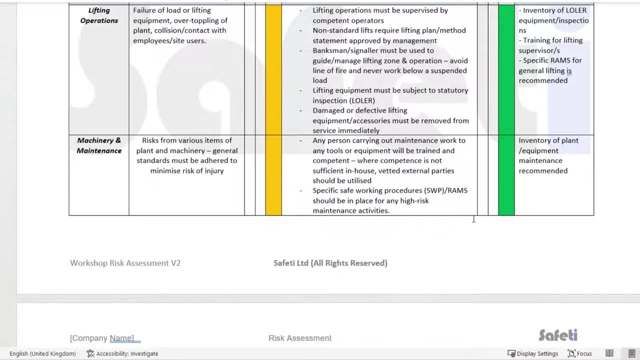 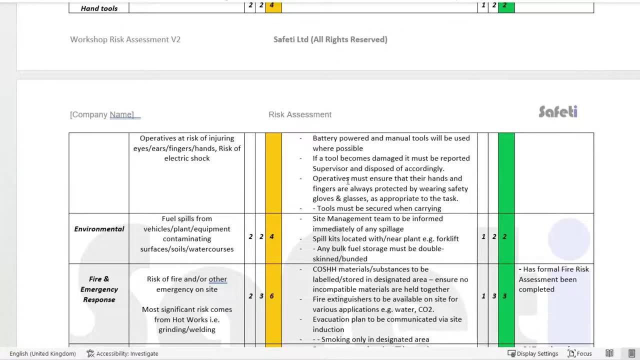 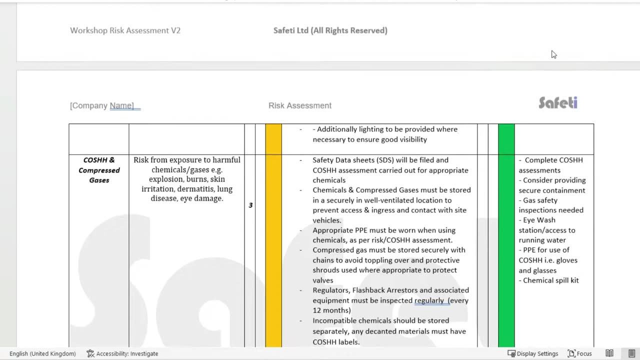 thrown in another one which is a slightly different risk profile, and again, you know lots of detail in this one as well. This one sort of crosses over with the construction end example that we have, and you can mix and match, of course. if you like this template better, you can. 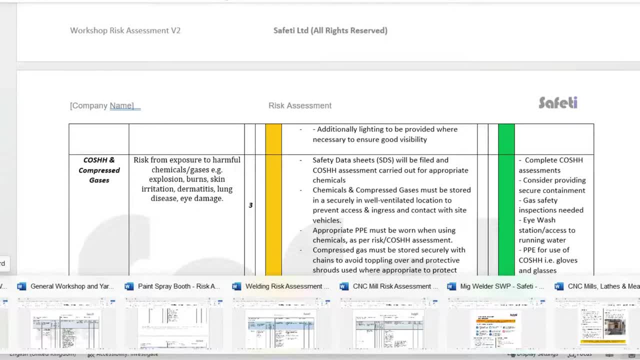 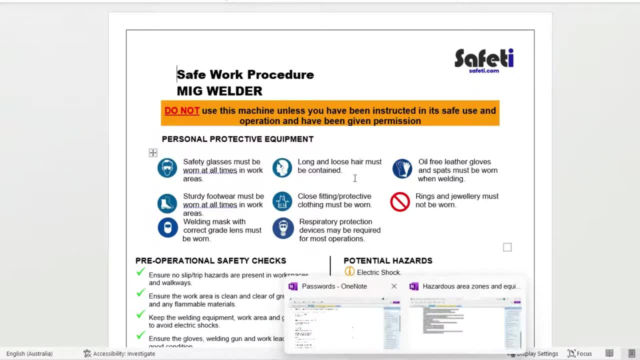 you can use it and bring the information across from the other one and vice versa, so it's up to you really. So just to make this a lot more valuable for you, and on top of that we've put in some free, safe work procedure examples which are- they're really one-page communication examples. 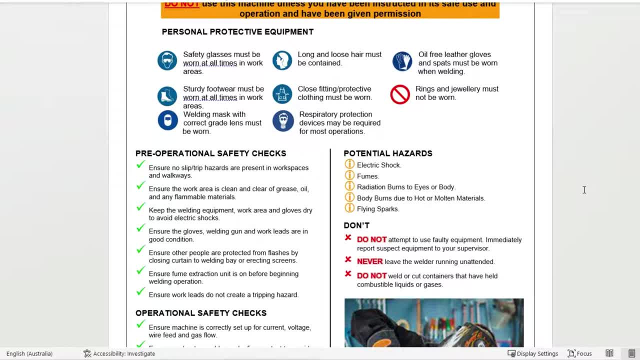 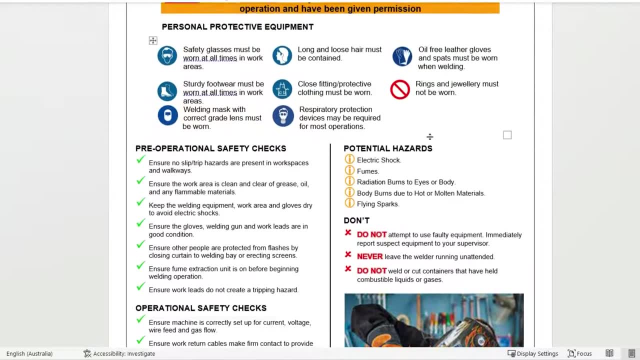 which can be posted or communicated as part of toolbox talks, emails and that type of thing, or just as part of general training. So, as you can see, quite a lot of detail on these as well, a bit of sort of pictogram use and sort of do's and don'ts. 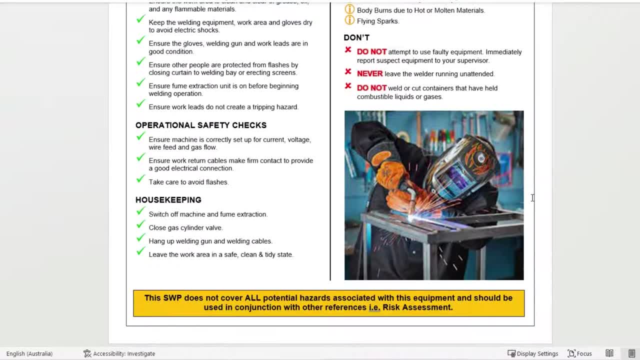 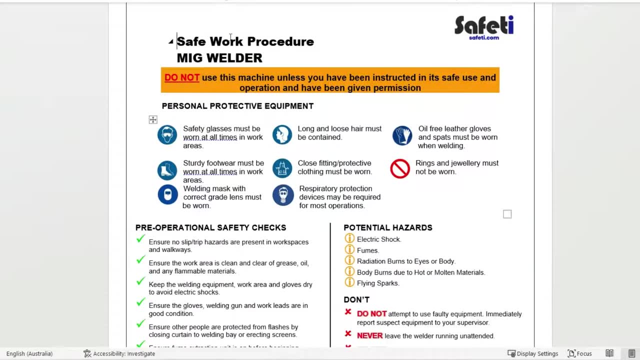 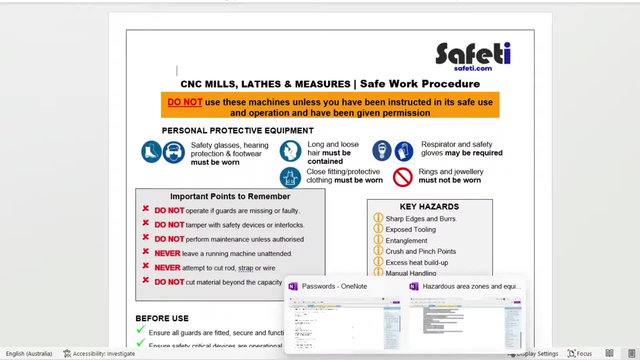 before, during and after guidance and general hazard guidance. so that kind of summarizes the risks and control measures for things like MIG welding there, as you can see. So there's five of those thrown in, including CNC mills- and lathes is covered as well- and air compressors- portable air compressors, which most workshops will. 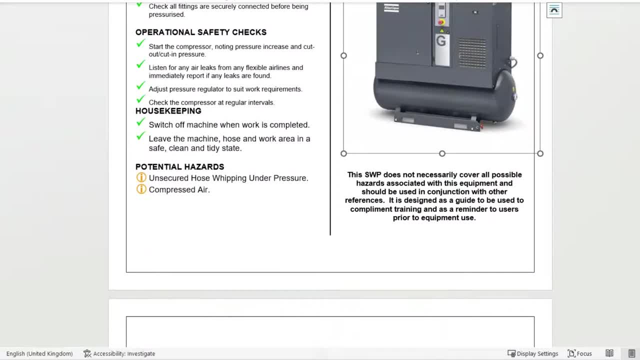 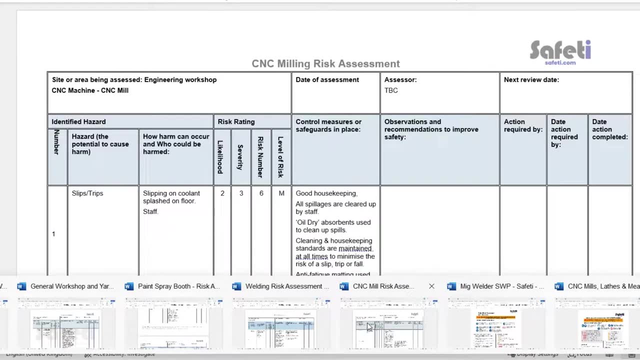 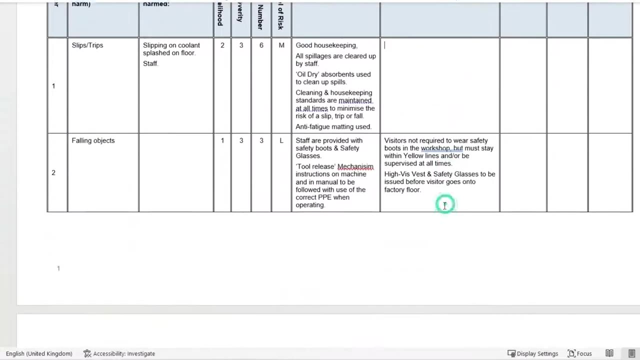 have as well. so hopefully again, those are really useful for you if you're working in an engineering workshop or workshop type environment. and to add even more value in, we've thrown in to this the CNC mill risk assessment, which again would apply to a lot of people that I'm not going to. 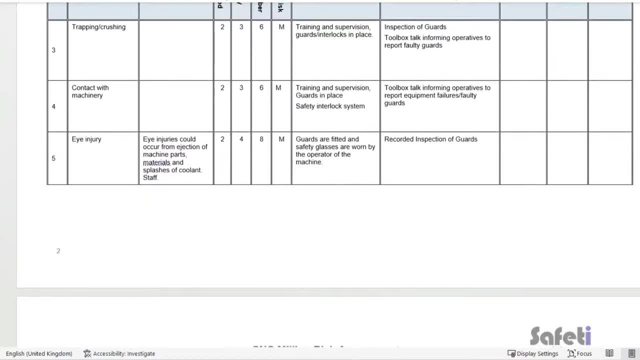 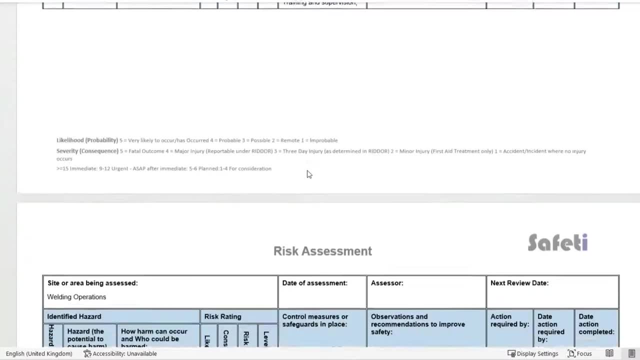 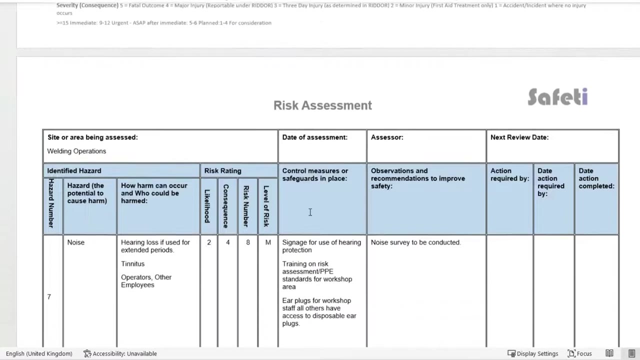 too much detail here, but that's a five-page assessment on, on its own, The welding risk assessment, which is really important. at the moment there's a lot of focus on control of welding fume and from the HSE and regulators in the UK certainly. so that is. 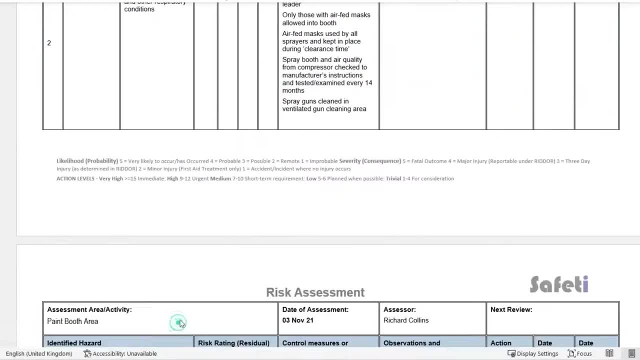 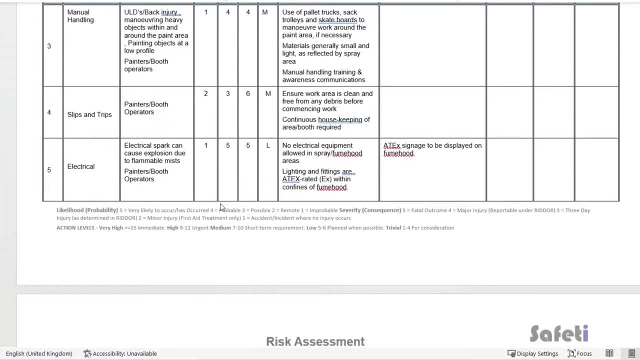 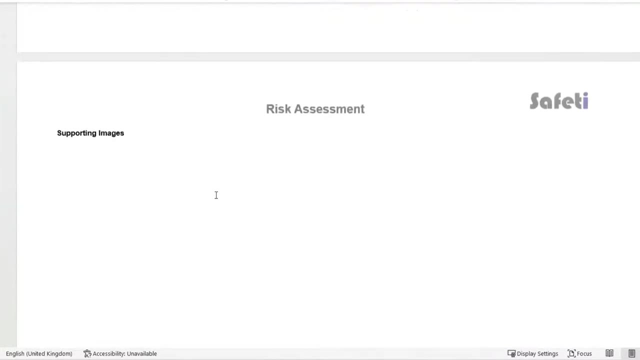 something that should be useful. that's another detailed document and, as well, we have a spray booth one that, again, I think, with a lot of our customers, certainly many of them will be doing some form of spraying in their facilities, so that hopefully, is is another useful five or six page document there for you.